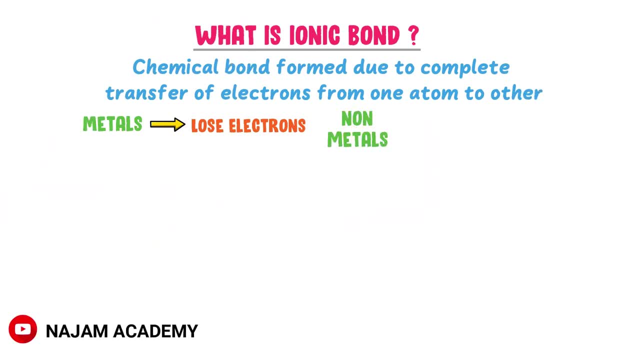 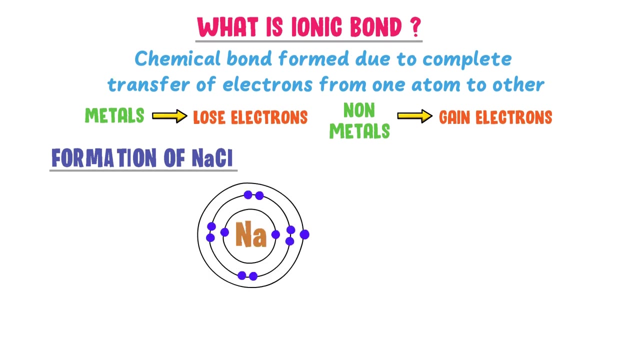 A solution that can be used to complete transfer of electrons from one atom to other atom is called ionic bond. Noted down that metals having low ionization energy- Here in this ionic compound, sodium is metal and chlorine is non-metal. 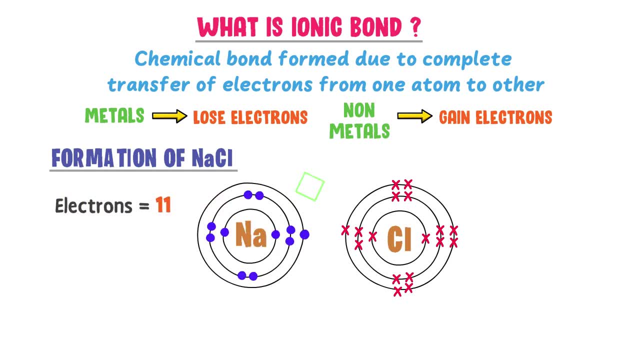 The total number of electrons in the sodium atom is 11 and the total number of electrons in the chlorine atom is 17.. Remember that in the Levy structure we represent the electrons of one atom by the dot and the electrons of other atom by the cross. 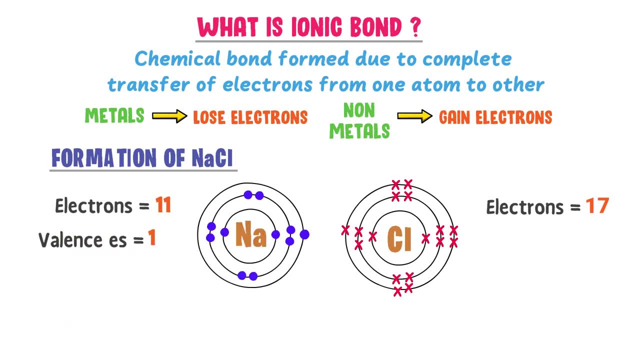 In sodium atom. there is only one electron in the outermost shell. We call it valence electron And the chlorine atom. there are seven electrons in the outermost shell which we call valence electrons. Now listen carefully. if sodium loses this valence electron, it will get stability because 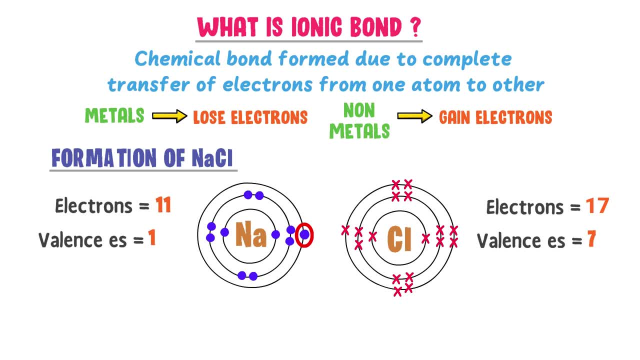 it's octane, The octet rule will be fulfilled. Secondly, if chlorine gains one electron, it will also get stability, because its octet rule will be fulfilled. Thus, sodium loses this one electron, our valence electron, and chlorine gains this. 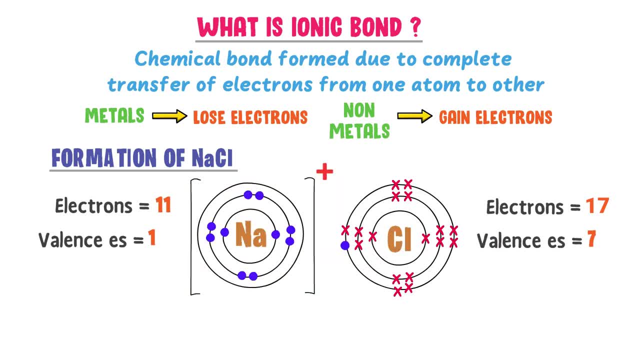 one, electron, Sodium, becomes positive ion, our cation, and chlorine becomes negative ion, our anion. These both ions have now opposite charges, due to which electrostatic force produces between them. This electrostatic force generates ionic bond between them. 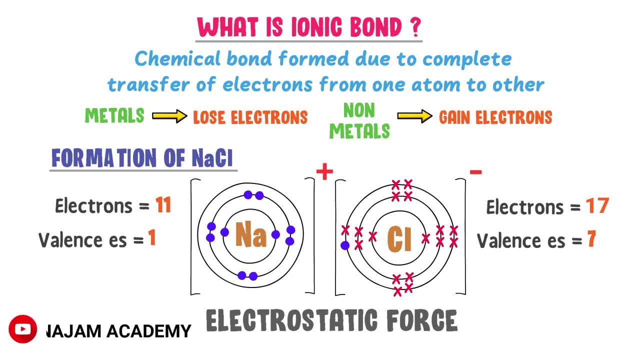 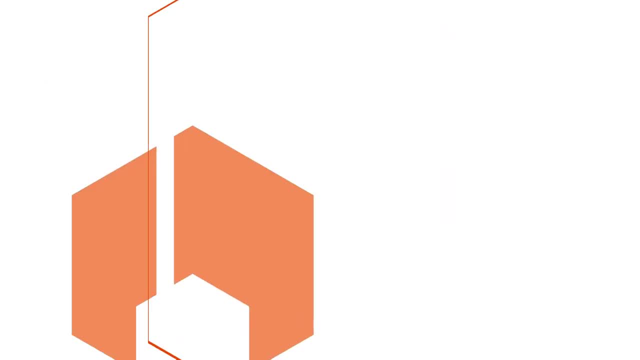 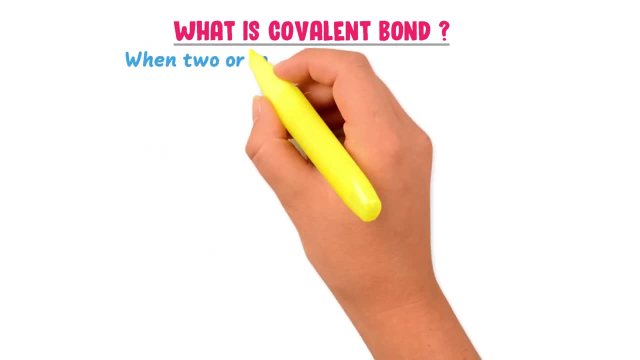 Therefore, we say that ionic bond is formed when metals lose electrons and nonmetals gain electrons. Now, what is covalent bond, Or how we define covalent bond? Well, when two or more atoms join together by mutual sharing of electrons is called covalent. 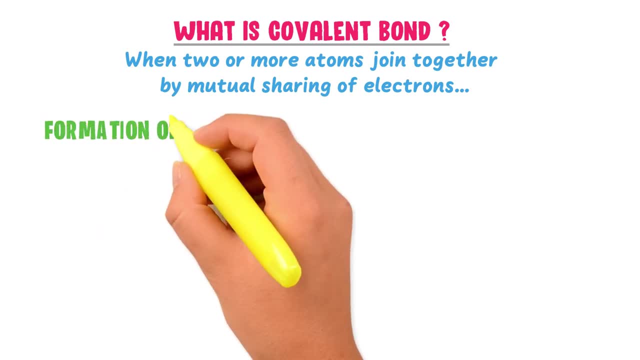 bond. For example, consider the formation of oxygen gas. Here let me write one oxygen atom and another oxygen atom. We know that the total number of electrons in single oxygen atom is eight and the valence shell of oxygen atom There are six electrons.